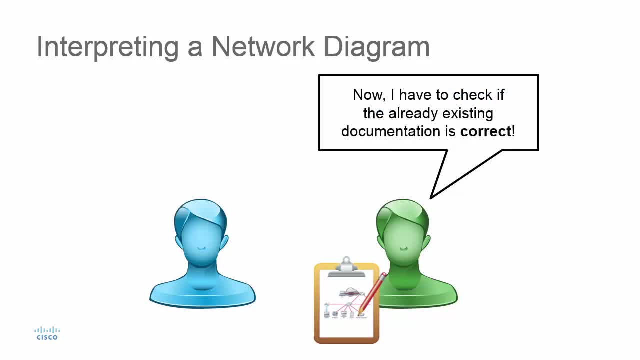 correct, And usually documentation isn't purely a representation of the physical topology or the logical topology, but it's usually something in between. Which map of the network will you use when you try to troubleshoot an IP phone connection somewhere in the network? 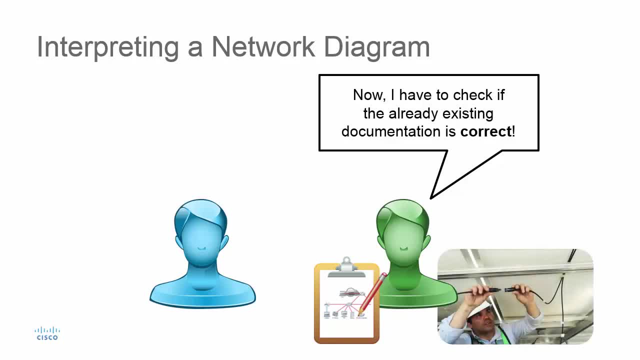 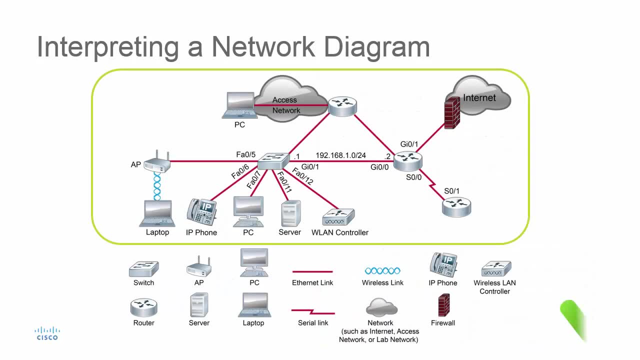 You don't need the exact path of a cable through the hallway. However, it is good to know on which port on a switch that cable connects to, And that's where a network diagram comes in handy. Well, based on the information that you have, can you guess what we represent? 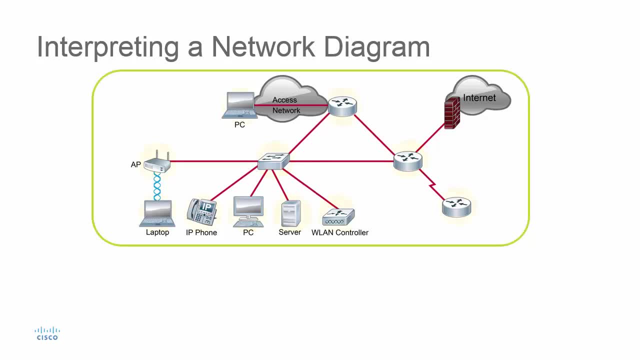 in our network diagram. First, different network devices. of course, When looking at the network diagram, you can find several icons depending on the devices that you have in your network: PCs, IP phones, wireless LAN controllers, routers, servers, firewalls and so on. 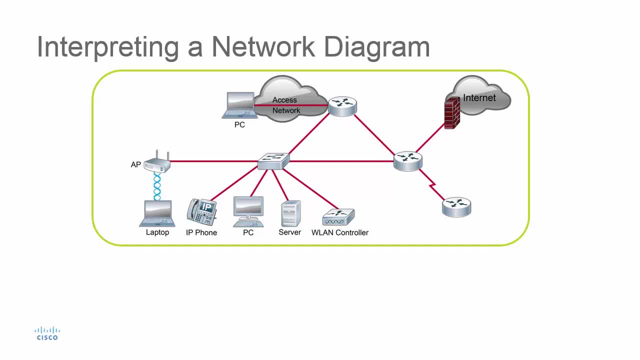 But if you had only devices on the diagram and nothing else, this information wouldn't be useful, right? If we go back to our previous example of troubleshooting an IP phone connection, how would you determine to which switch this port is connected to? For this reason, besides devices, we also include other information on this network diagram. 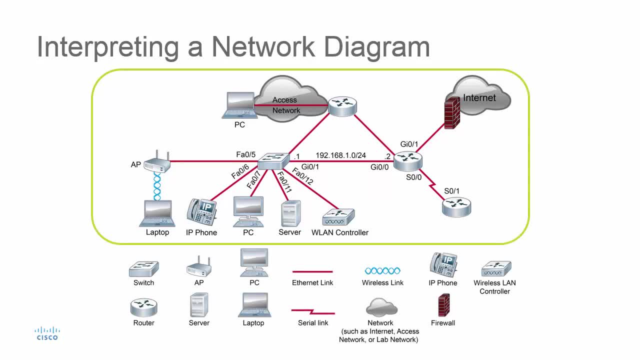 Combining all that information is what makes the network diagram really useful. So it's common to identify the interconnections between devices along with the interface identification. If you take a look at our network diagram, you can see different interface identifications. S0- slash 0 is a format used for a serial interface. 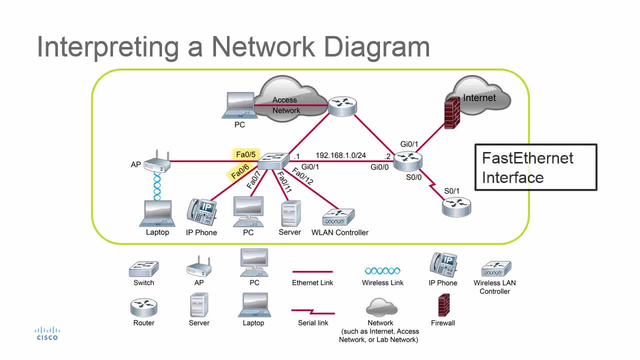 Can you name any other? You see FA0 slash 5 or FA0 slash 6 and so on. right, Those are formats used to identify fast Ethernet interfaces. You can also see GI0 slash 0. And GI0 slash 1.. 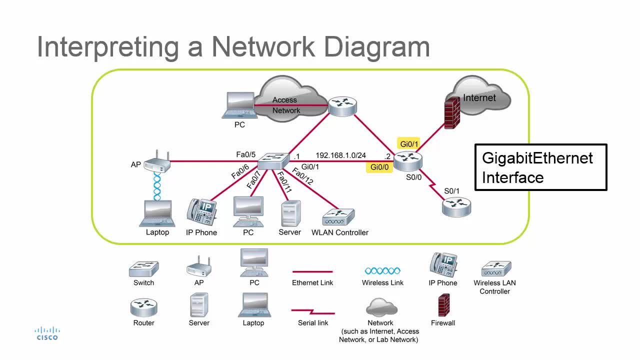 Can you guess what those are? Yes, they're identifications for gigabit Ethernet interfaces. Besides the interface identification, it is common to include the network address of the segment on the diagram. In our example you can see the 192.168.1.0 slash 24 network segment. 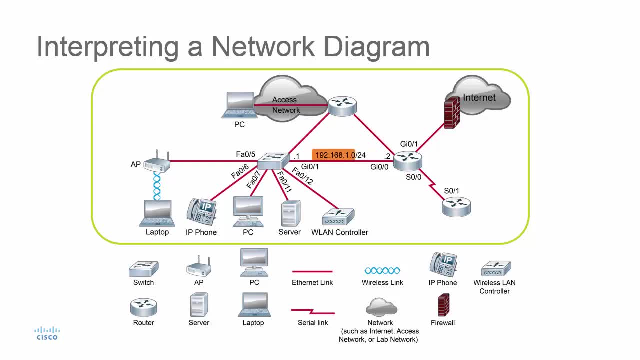 Here the IP address 192.168.1.0 indicates the network address and the slash 24. Indicates the subnet mask. But the network segment as such doesn't tell you much, So you normally include also the exact IP addresses on the interfaces.